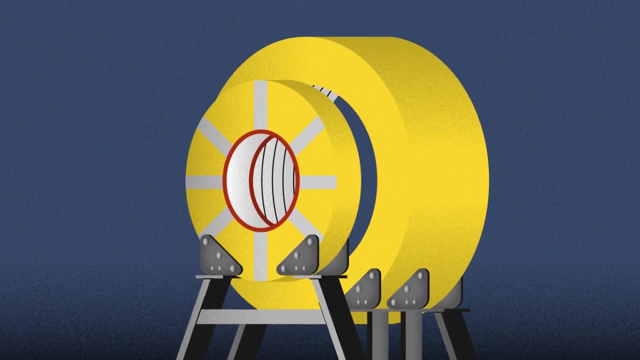 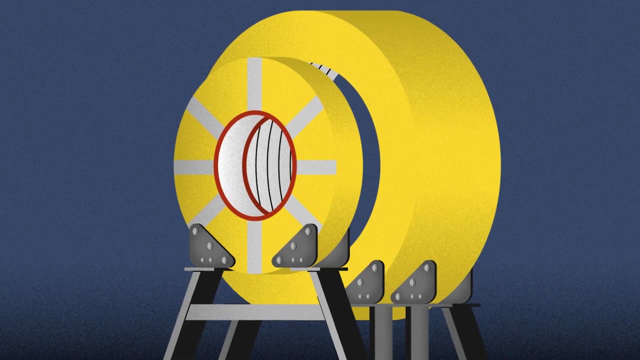 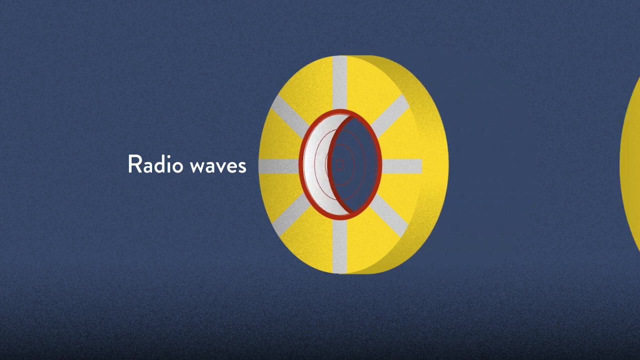 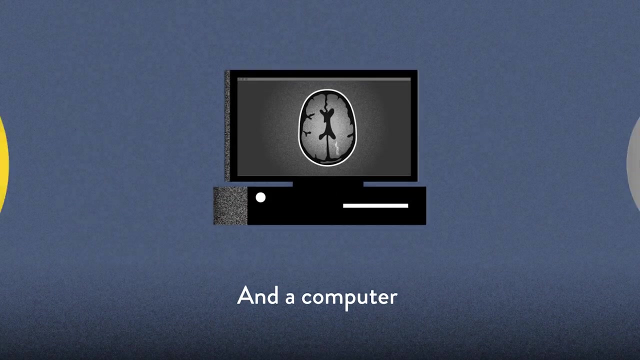 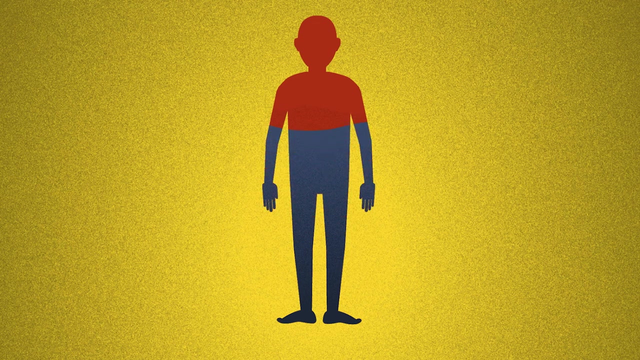 MRI is a medical imaging device commonly used to examine the soft tissues of the human body. Let's meet the machine. The key components are the magnet radio waves gradient and a computer. Our bodies are made up of 60% water, and water is magnetic. 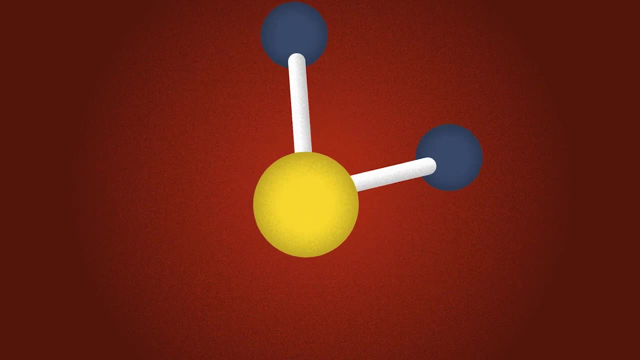 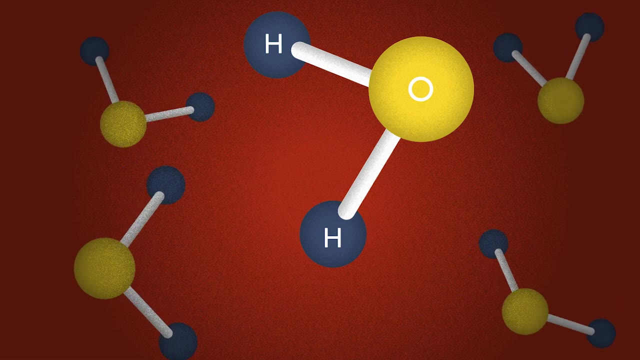 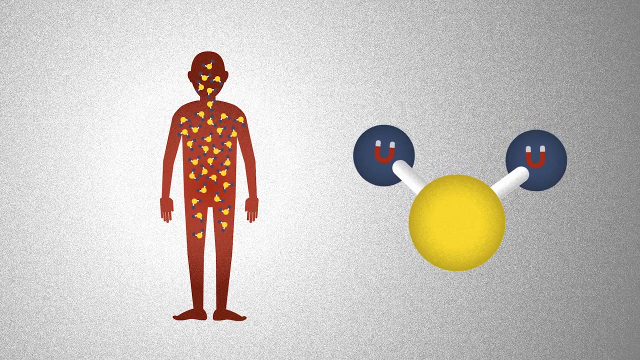 Each of the billions of water molecules inside us consists of an oxygen atom bonded to two hydrogen atoms. We know it as H2O. Small parts of the hydrogen atoms act as tiny magnets and are very sensitive to magnetic fields. MRI stands for Magnetic Magnet. 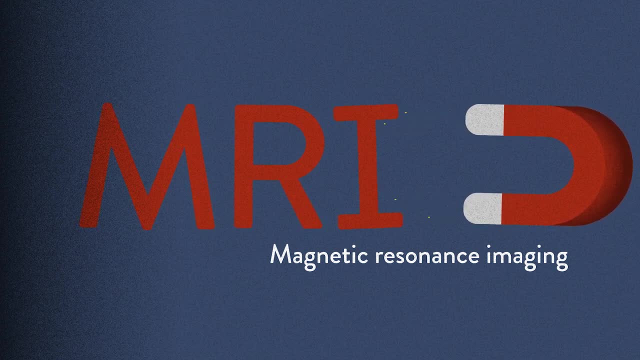 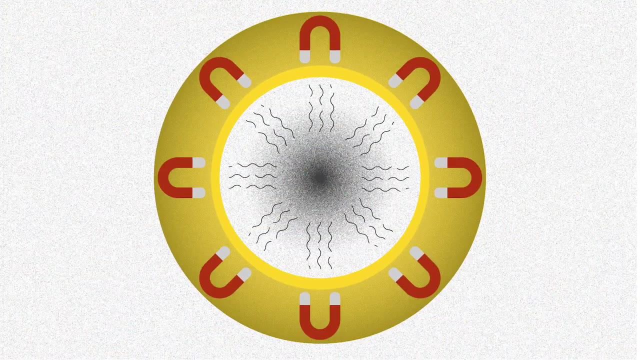 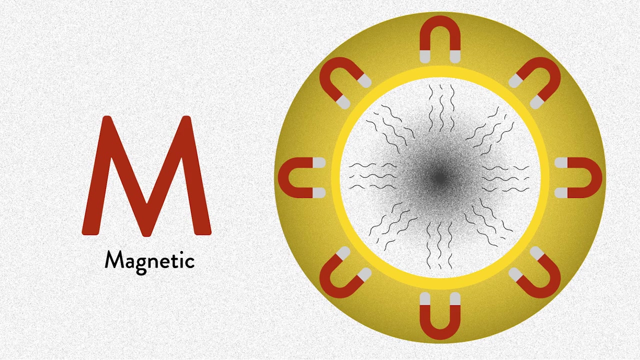 Magnetic Magnet stands for Magnetic Resonance Imaging, and an MRI scanner is one of the main diagnostic tools that doctors use to examine inside our bodies. The first step in taking an MRI scan is to use a big magnet to produce a unified magnetic field around the patient. 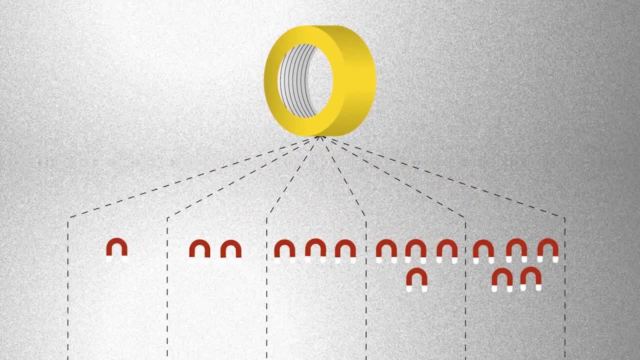 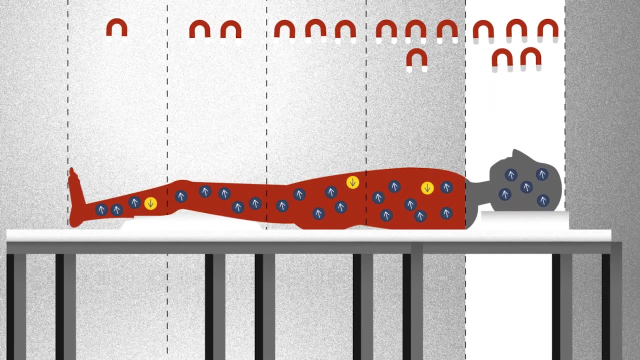 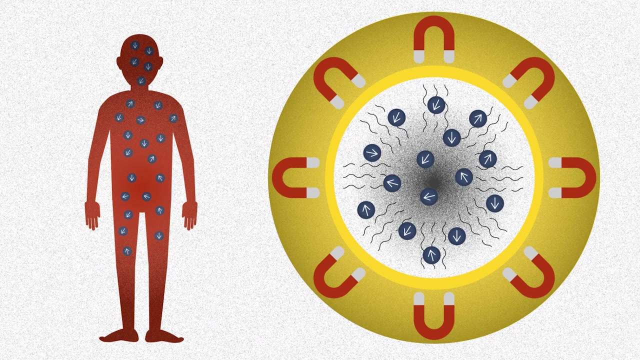 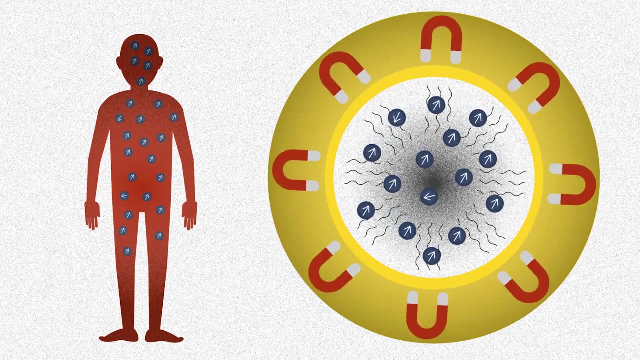 The gradient adjusts the magnetic field into smaller sections of different magnetic strengths to isolate specific body parts, For example the brain. Normally the water molecules inside us are arranged randomly, but when we lie inside the magnetic field most of our water molecules move at the same rhythm or frequency as the 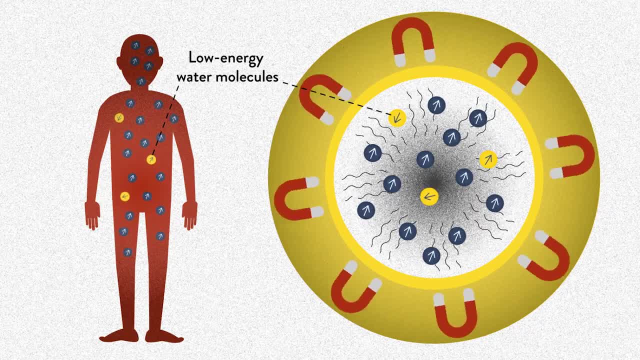 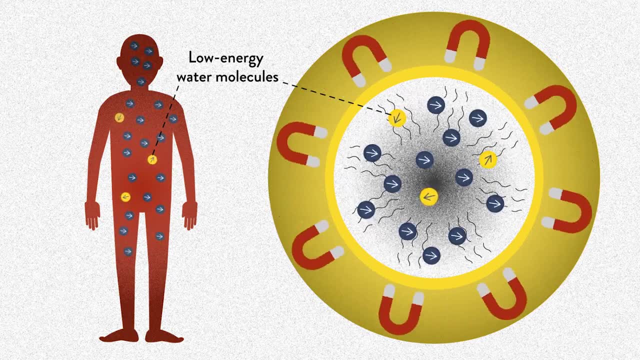 magnetic field. The ones that don't move along the magnetic field are called low-energy water molecules. To create an image of a body part, For example the brain, the brain, the machine, focuses on the low energy water molecules. Radio waves move. 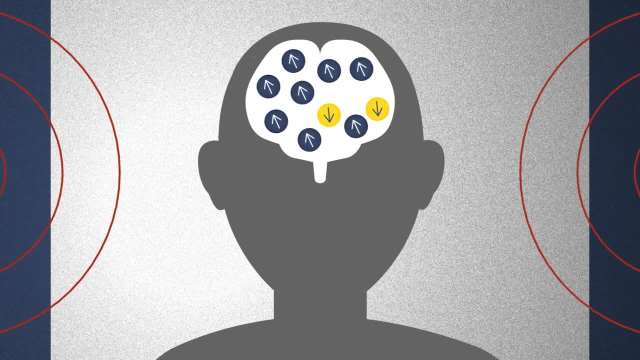 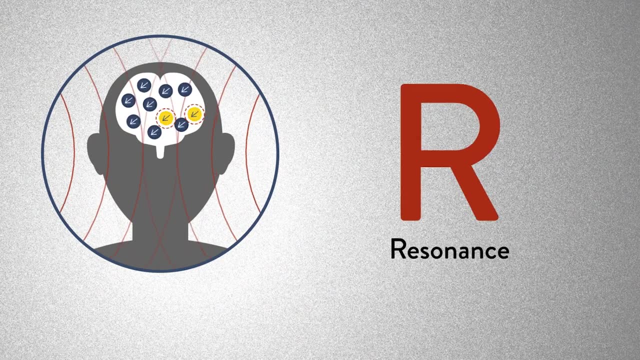 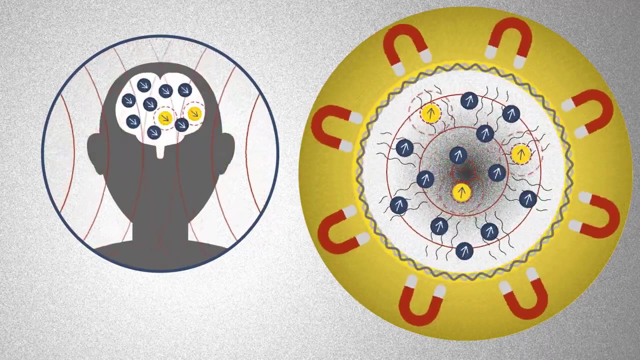 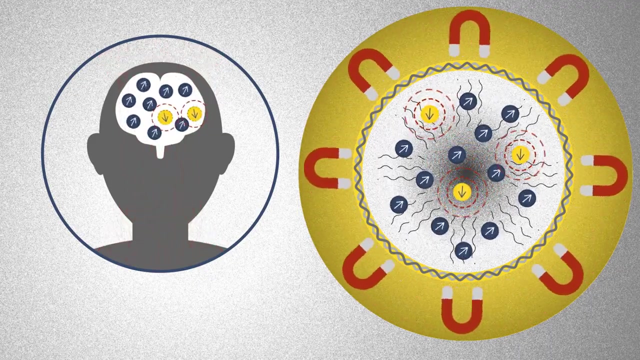 at the same rhythm or frequency as the magnetic fields in an MRI machine. By sending radio waves that match or resonate with the magnetic field, the low energy water molecules absorb the energy they need to move alongside the magnetic field. When the machine stops emitting radio waves, the water molecules that had